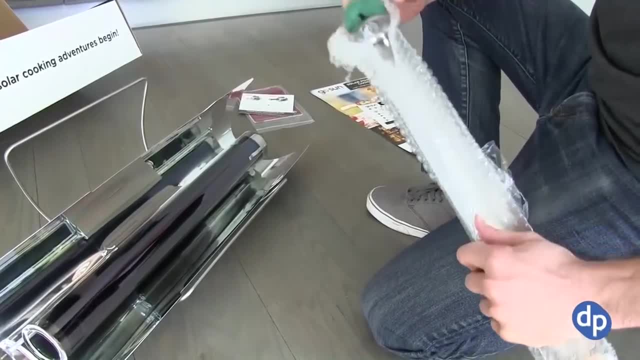 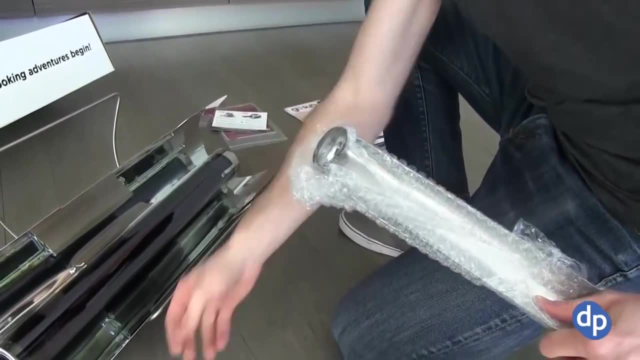 I did. Yeah, the whole thing is almost completely assembled already. really, You just have to do a little bit of unwrapping, pull some plastic off and turn the handle around on one thing: Yeah, you're done, That's it, And it's so. the just weirdest thing about it is you put this thing. 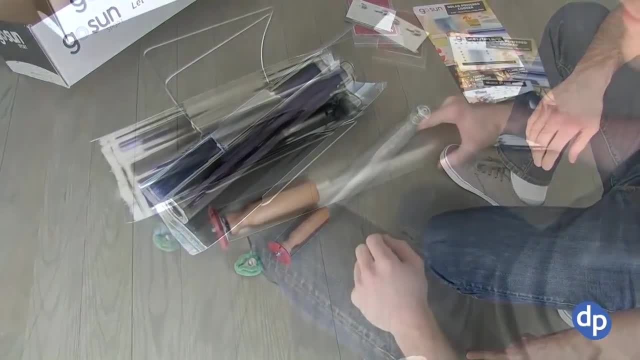 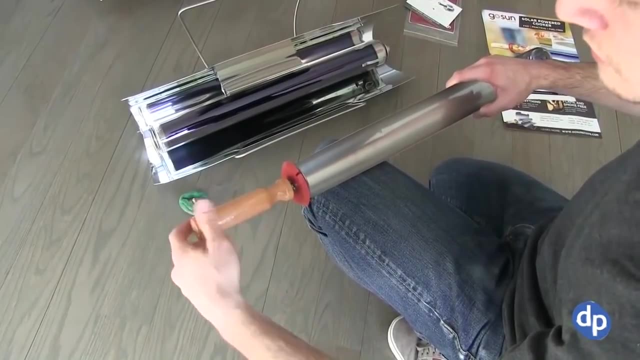 together. There's no plug, There's no place to connect a gas line or propane or oil or whatever the case may be. You basically just set up the handle for the food tray. As you can see, the food tray on this one. this is the sport, so it's not huge, but you can still fit. 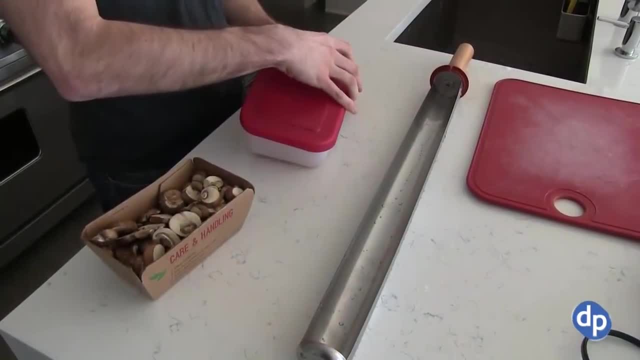 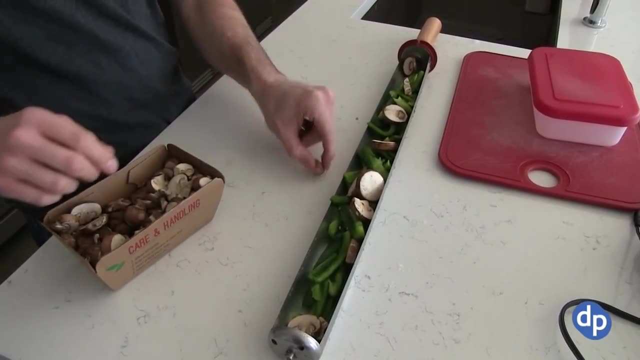 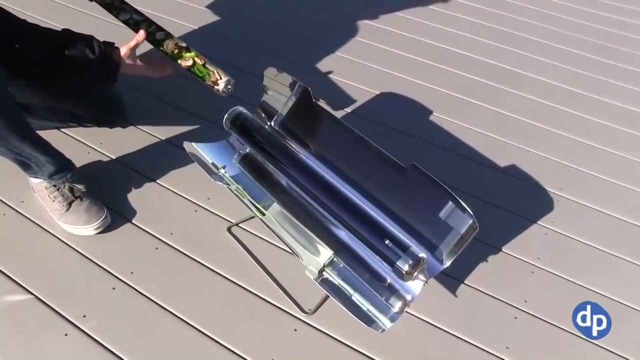 quite a bit of stuff in there. We put that together and we were essentially ready to go. I loaded it up with much to Lewis's pleasure, not only green peppers but also mushrooms- mushrooms, one of Lewis's favorite vegetables and just a very compelling vegetable to Lewis. We set 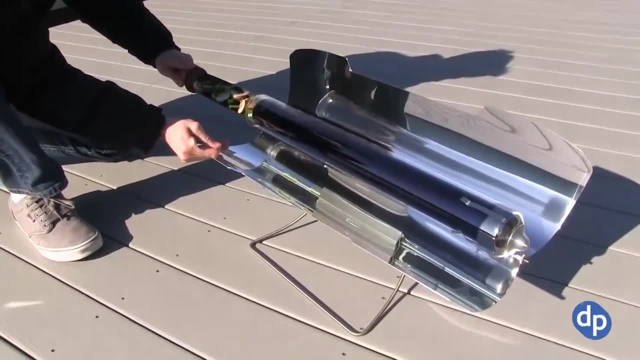 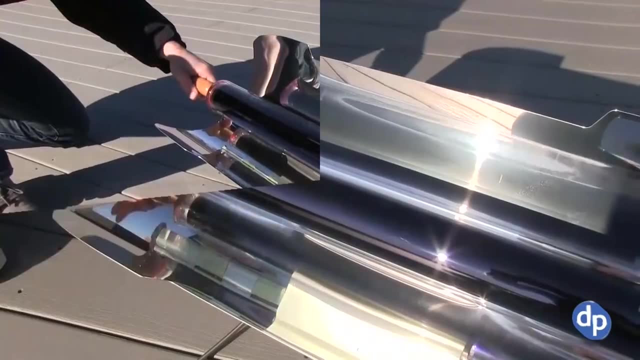 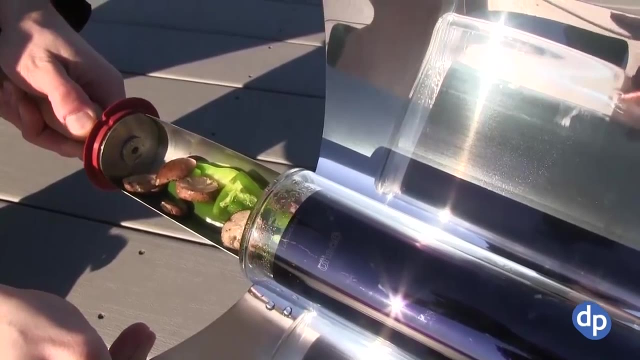 up the food tray. I completed the assembly, inserted the food tray And then the trick to it is: you want to sort of align these reflectors so that the sun is directly aimed at the food. And as you see me opening it, it's steaming, Lewis, I mean it is. we just left it in the sun 20 minutes. 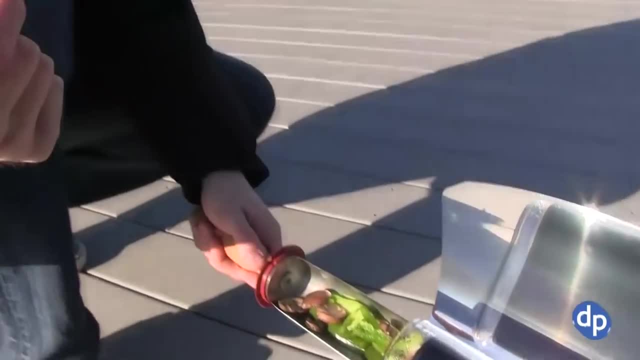 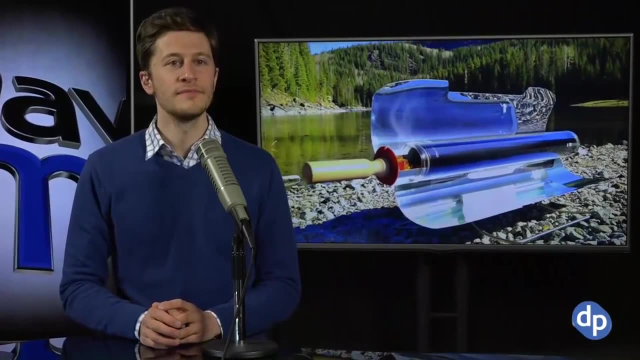 and the food was hot to the touch and steam coming out of it. Truly amazing, isn't it? Speaker 1. It is, Yeah, Dave. you see, Dave kind of burned his finger a little bit there. Speaker 2. On that, on that stove. Now, I am not really someone who goes camping. 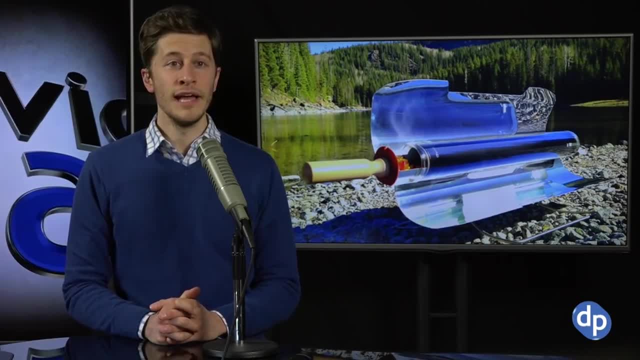 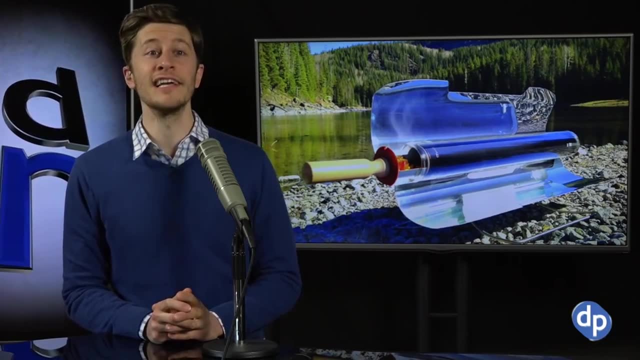 Lewis's last camping attempt ended up with him in a hotel and visiting four star restaurants in Portland Maine. So maybe neither one of us really are the best campers, But if you were to go camping again, Lewis, you'd be totally up for bringing something like this. Yeah, it is, It is. 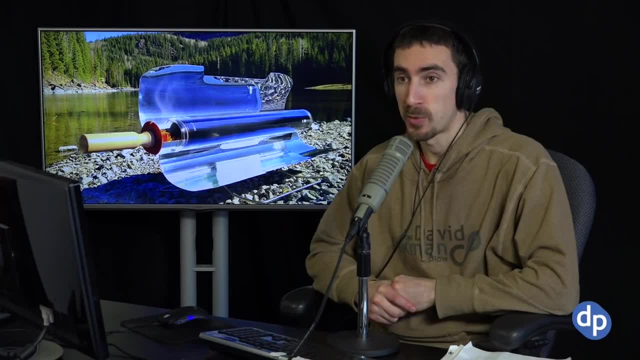 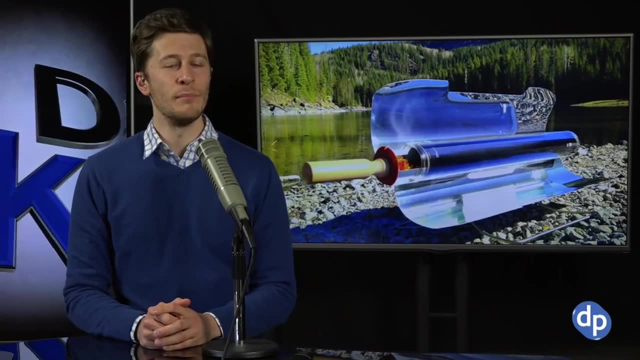 a great product And it really works. the same way those solar farms work. You focus the lights on a tube, use the sun's power, cook stuff. Speaker 1: You were to bring if you were to have the bigger version right, because this was the sport. So 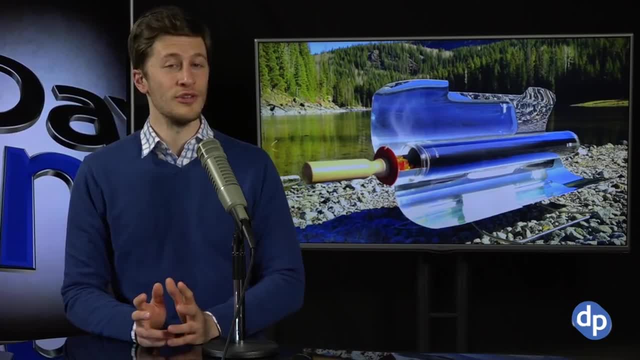 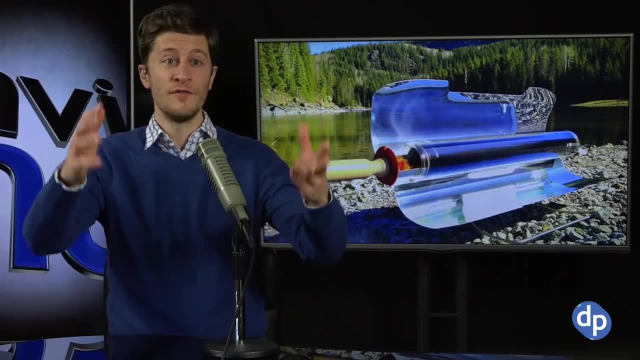 the food tray is not huge. They make bigger ones when you can. you can actually cook like three pounds of meat in one sitting. Is that appealing to you, The idea of being able to just pull this thing out and cook meat? or even that you could go fishing and catch a fish and then with no